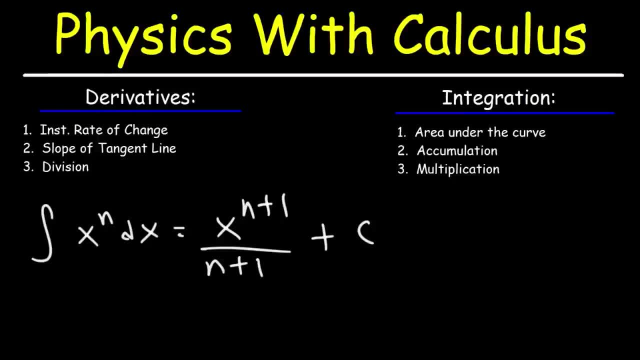 So when you integrate, you're going to introduce a constant. So let's put this into practice. What is the antiderivative or the indefinite integral of x cubed dx? So this is going to be x to the 3 plus 1, divided by 3 plus 1, plus c. 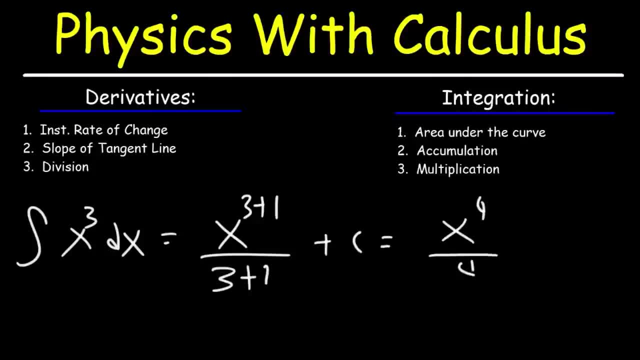 So this ends up being x to the 4th divided by 4 plus c, And so you can write that as 1, 4th x to the 4th plus c. Now let's try another example. Let's find the indefinite integral of 7x to the 5th power. 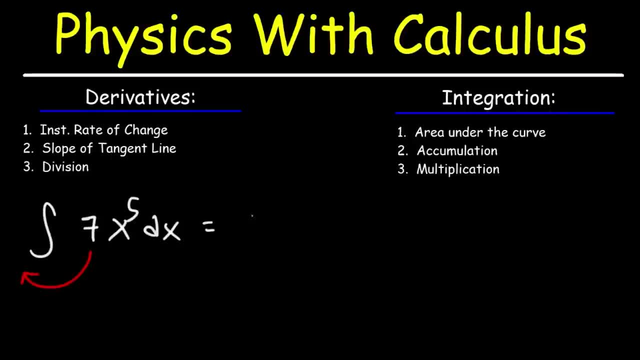 So for this example, you could take the constant and move it to the front. So this is the same as 7 times the integral of x to the 5th, power dx. Now, using the power rule for integration, the antiderivative of x to the 5th is x to the 6th divided by 6.. 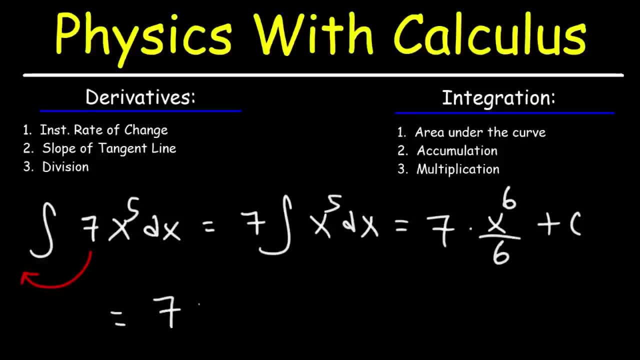 And then plus c. So our final answer is 7.. You could say 7 over 6 times x to the 6th plus c. Now I want to talk about the relationship between derivatives and division with that of integration and multiplication. 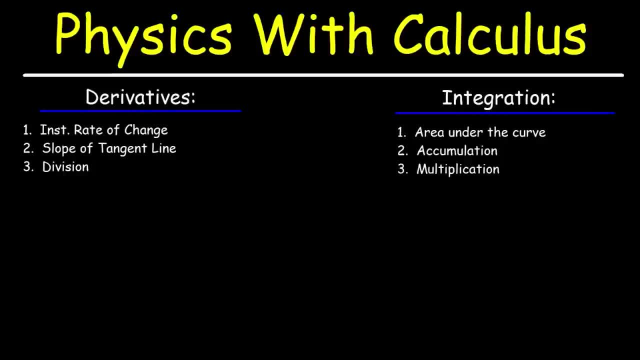 So in physics, sometimes you may have a simple formula to deal with. Other times the formula might involve calculus. For instance, work is the product of force and displacement. Now, displacement could be in the x direction or it could be in the y direction. 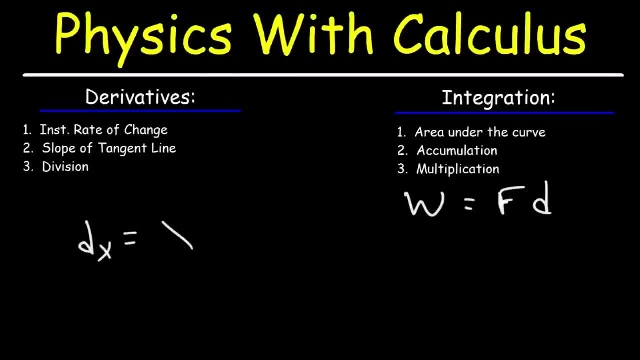 In the x direction displacement, you could simply call it x. In the y direction, it's really just y. Well, technically it's the change in x or the change in y, Because displacement is the final position minus the initial position. 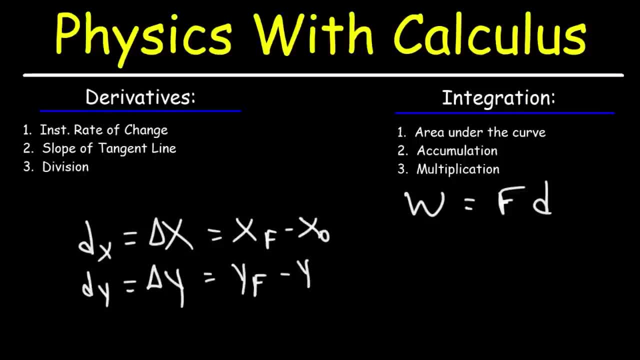 So this is the final position. So this is the final position, minus the initial position. It could be along the x axis or along the y axis. So whenever you see d, it represents displacement. Now this formula should be applied if the force acting on an object 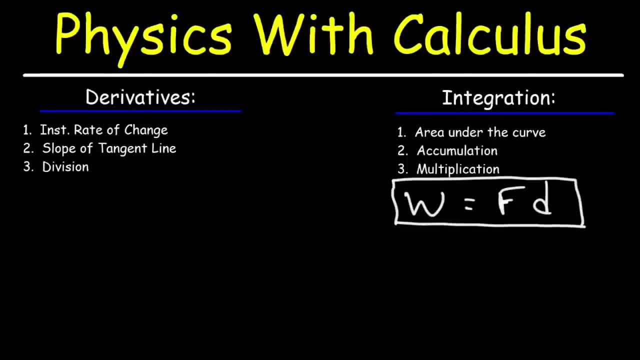 that is, the net force is constant. But what if the net force is not constant? What if it varies based on the displacement? What if it changes? In this case, you need to use calculus. Whenever something is not constant, you need to use calculus to get the answer. 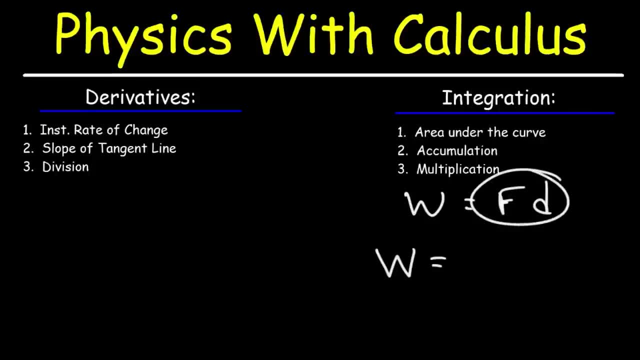 Notice that the force is being multiplied by the displacement. It turns out that the work done by a variable force is the integral of that force, or let's say that force is a function of the displacement along the x direction, times, dx. Now you're going to integrate it from a to b. 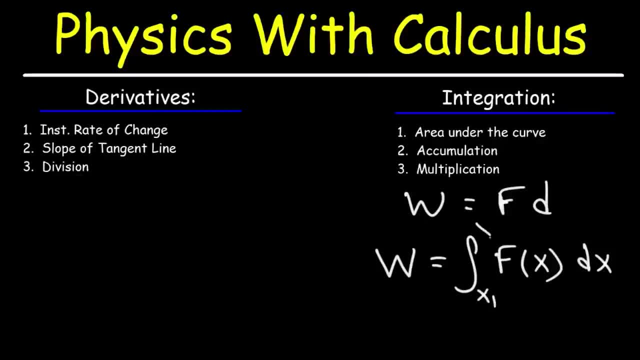 So a and b will be like an x value. Basically, x1 will be the initial position, x2 is your final position. But what I want you to realize is that when you have a formula, if you're multiplying two variables, 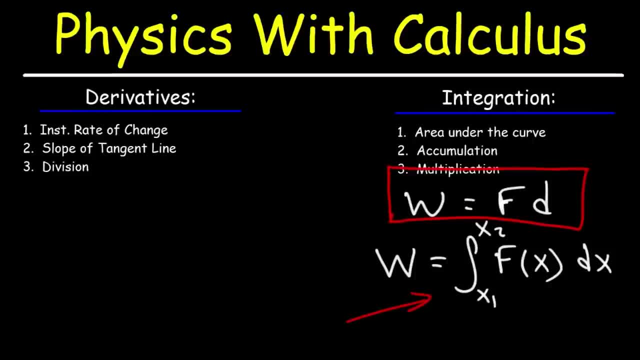 that formula is going to be associated with integration. When you're dividing two variables, that formula will be associated with differentiation or derivatives. So let me give you another example. Average velocity, which I'm going to represent like this, is basically the change in position or the displacement over time. 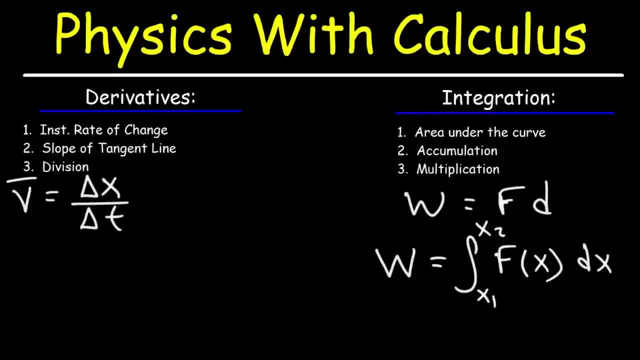 So we're dividing displacement and time. So this formula is going to be associated with derivatives. It turns out that the instantaneous velocity as a function of time is the derivative of the position function with respect to time. So, as you can see, you need to associate division with differentiation. 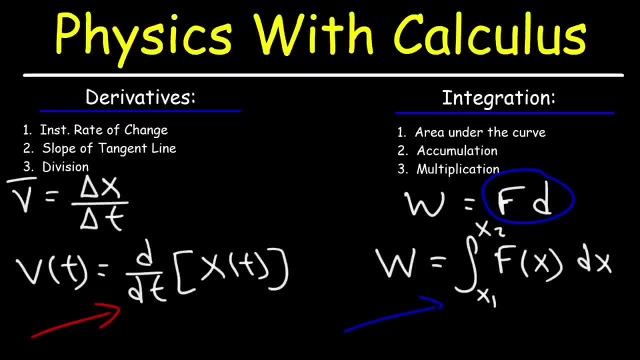 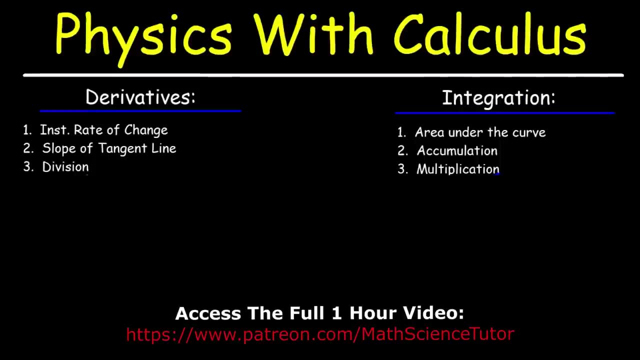 and associate multiplication with integration. Now let's see if you got the point that I'm trying to make. Let's start with a function of time. Let's start with a familiar formula. In your physics textbook you'll see this formula. 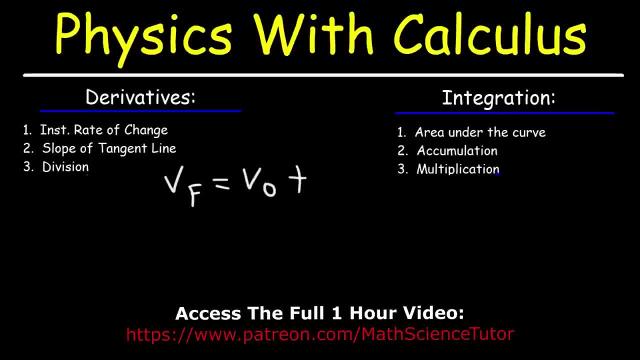 Final velocity is equal to the initial velocity plus acceleration. Now, with this formula, there's a lot of things we can do. Here's one thing I'm going to do: I'm going to move the initial velocity to the other side. So I have v final minus v initial is equal to at. 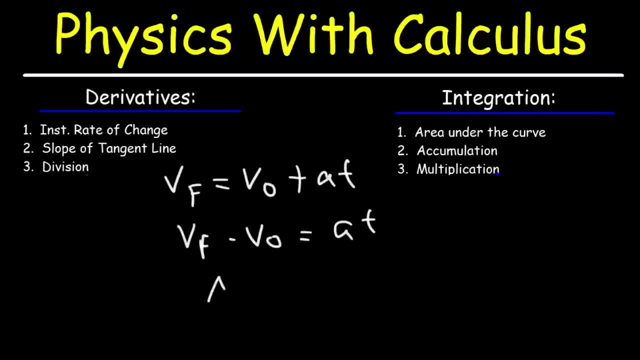 Now this represents the change in velocity. So I'm going to represent that as delta v, Where delta means change. So I get this formula: The change in velocity is equal to the acceleration multiplied by the time. Now let's save that formula. 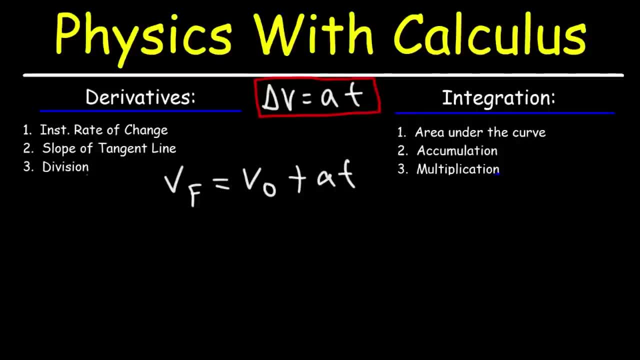 We'll talk about it later. Now, starting from the original formula that we have, let's solve for a, So I'm going to move this to this side. So once again, I have v final minus v, initial equals at. 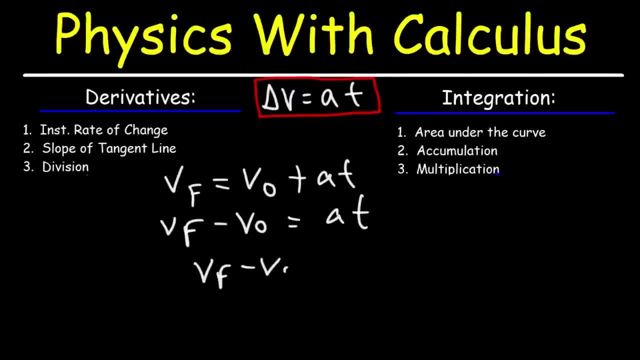 And then dividing by t, I have that. So I have v final minus v initial equals at, And then the acceleration is v final minus v initial over t, And we know this is the change in velocity. So we can say that delta v over, I guess you could say delta t. 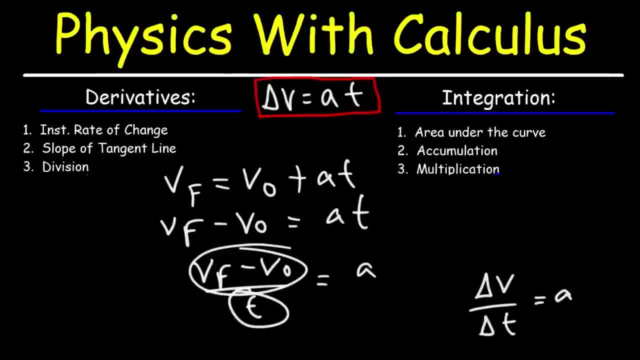 This t is really delta, t is equal to a. So, looking at these two formulas, which one is associated with derivatives And which one is associated with derivatives? So let's say, if we're focused on this formula, If the acceleration is constant, you can just use this formula to calculate the change in velocity. 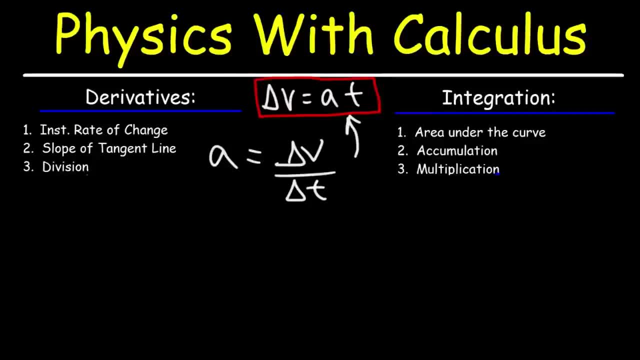 But let's say, if the acceleration is not constant, Let's say it's a variable, Would you use integration or differentiation to calculate the change in velocity? Notice that we're multiplying a by t, So that's going to be associated with the change in velocity. 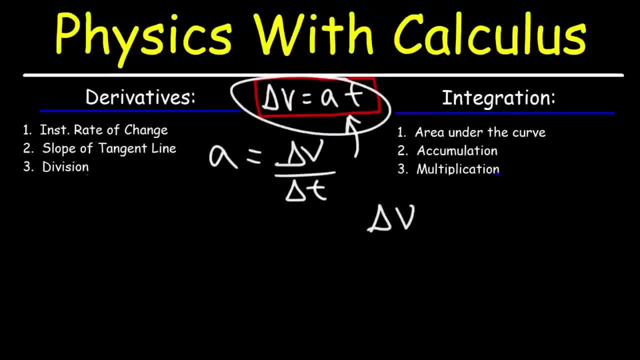 Thus, the change in velocity will be the integral of the acceleration function, where a depends on t, from t1 to t2.. From an initial time point to a final time point. Now let's think about what this means If we have a graph with the acceleration in the y direction. 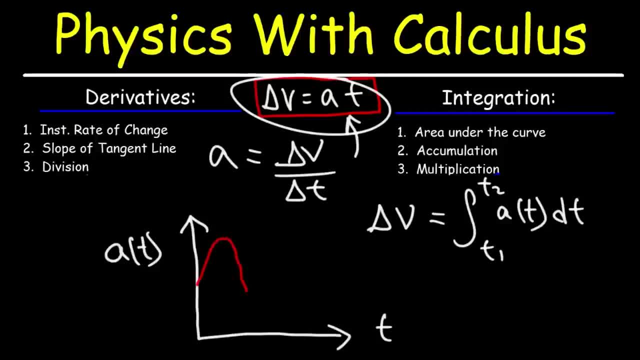 And time in the x direction. Now let's say the acceleration is a variable. We can calculate the change in velocity of the object, Let's say from t1 to t2 or from a to b, By finding the area under the curve. 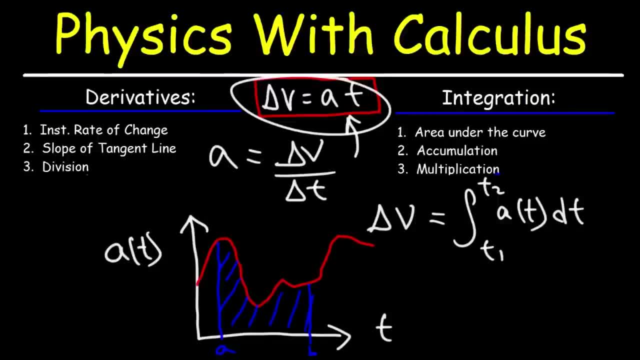 Now, sometimes you could use geometry to find the area under the curve. Other times you have to use calculus for a shape like this. But what you want to take from this is that The area under this curve highlighted in blue represents the change in velocity. 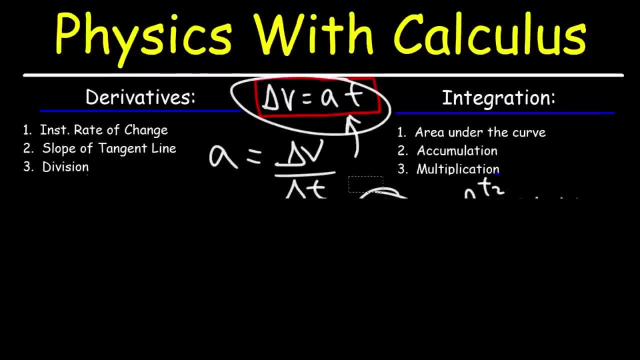 Likewise, if we go back to the other function where we said that work is the definite integral of the force When it's a function of x, If we graph this, where f is on the y axis, The displacement is on the x axis. 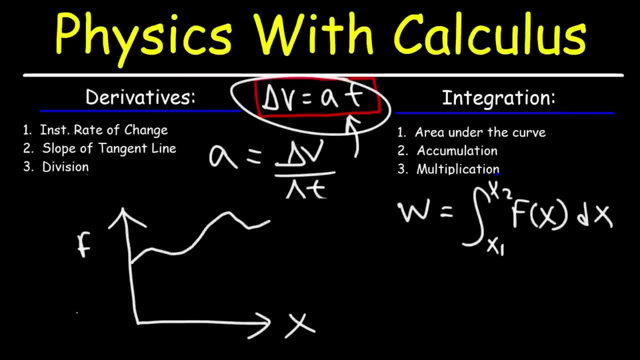 Now, let's say the force is a variable function. If we integrate it from a, let's say, to b, The area represented by the shader region is equal to the work done by the net force. So this is just not any force, but it represents the sum of the forces acting on the object or the net force. 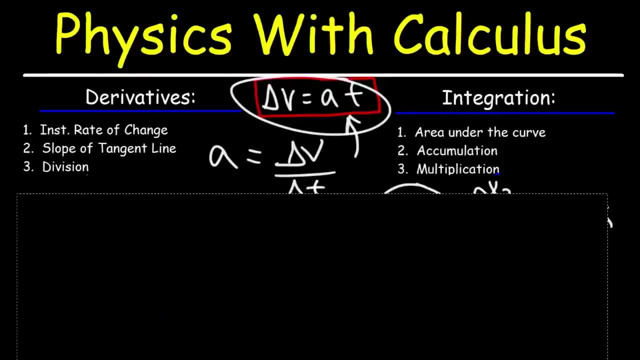 So make sure you keep that in mind. The area under the curve is associated with integration, Which is also associated with multiplication. When you wish to find the area of an object, let's say a rectangle- It's length times width. You're multiplying the length and the width. 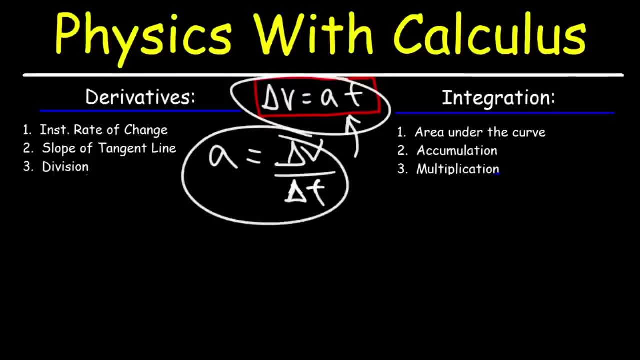 Now let's talk about this other formula. Acceleration is the change in velocity Divided by the change in time. So here we're dealing with division. So this tells us that acceleration is the derivative of velocity, It's the instantaneous rate of change of the velocity function. 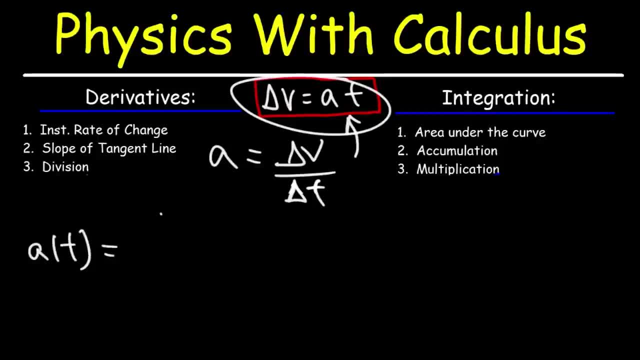 So if you wish to find the acceleration function, All you need to do is differentiate the velocity function with respect to time. Now let's draw a graph. Now let's say: this is the acceleration on the y-axis, Time on the x-axis. 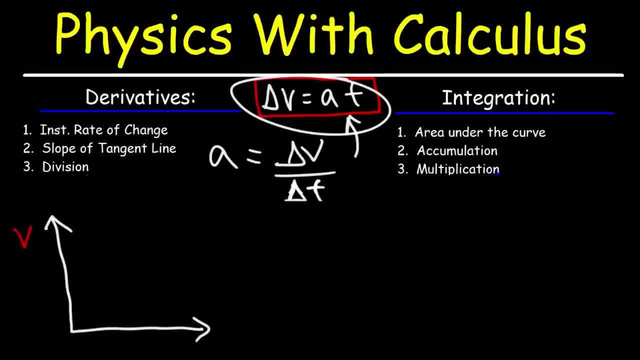 Actually let's use velocity. So velocity on the y-axis, Time on the x-axis. Now let's say the velocity is just, it varies, It's not constant. If you wish to find the acceleration function From the velocity,